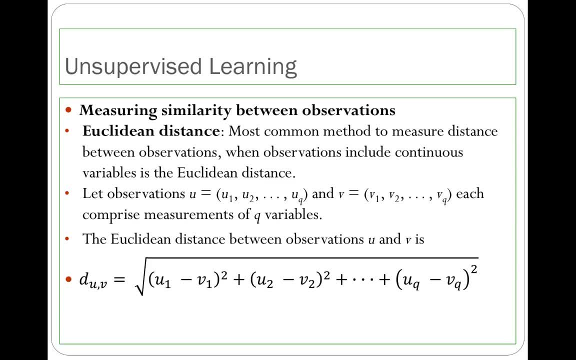 Also, another important point to remember is that one of the most important topics to review is the way that we calculate the distance between observations. If I have two observations, there are two methods that I can calculate the distance between the two observations. Suppose that the two observations are represented as u and v. 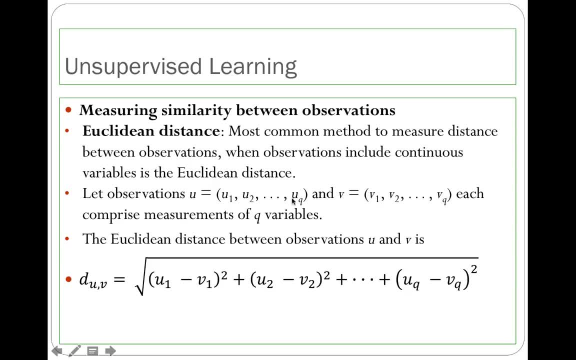 We show them as a vector u and vector v. If I want to calculate the distance between these two vectors, one simple way is the Euclidean distance, which takes the summation of the squared of the differences between each pair of the observations. So we can calculate the distance between the elements of the two vectors. 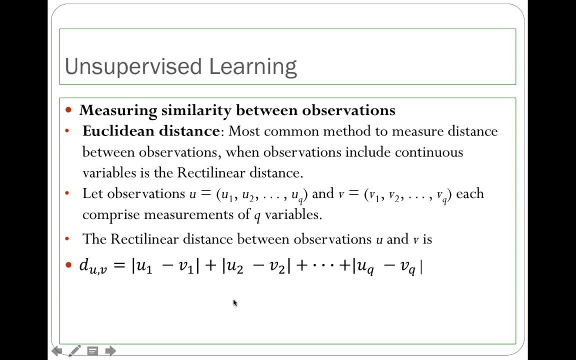 as shown below. here, Another measure of distance between the two vectors could be looking at the rectilinear distance between the two observations, which is basically: this time, instead of the sum of the squared differences, we simply take the sum of the absolute differences between the observations in each of these vectors. 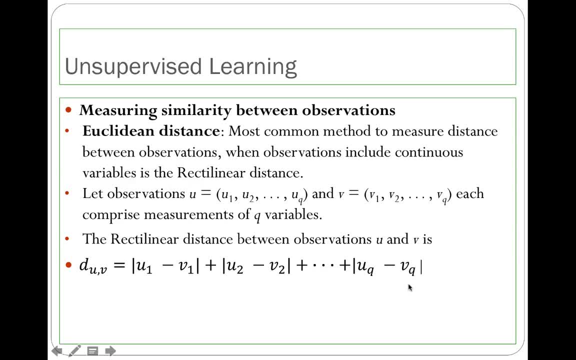 So this equation is presented here To see the application of rectilinear distances. in the example that we covered today, we're going to use rectilinear distances and you get a chance to see how we can use it for calculation of distance between observations. 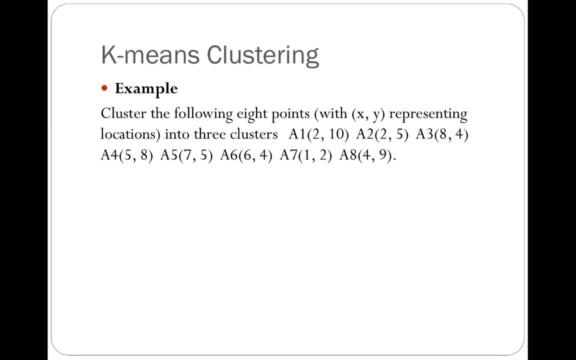 So let's look at one example and explain K-mean clustering with an example so that it's easier and more intuitive for us to understand. Suppose you have a two-dimensional set of observations, You have points, so you have eight points and all of them are two-dimensional. 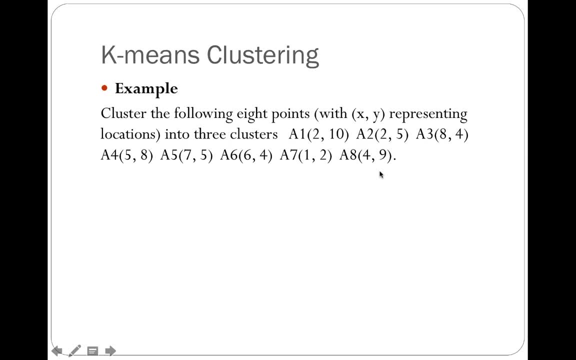 It means that it's in an x-y axis. so you have all these information here and you would like to cluster them in three groups. So one of the criteria or one of the parameters of K-mean clustering is number K. K refers to the number of groups. 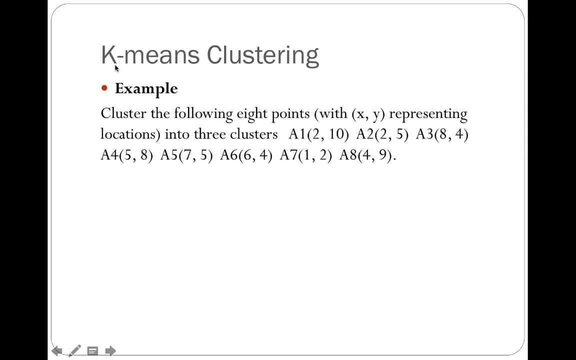 Despite the hierarchical clustering that we saw earlier, where the number of groups were not identified or determined before the clustering. in K-mean clustering you have to know what K or the number of groups are. In this case, the number of groups are three. 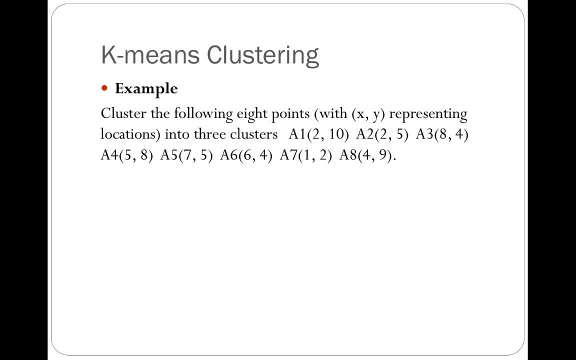 or we want to cluster the data points in three distinct groups. To start the K-mean clustering, we have to have a center for each of these clusters. It means that since K is equal to three, I have to identify three center points for these clusters. 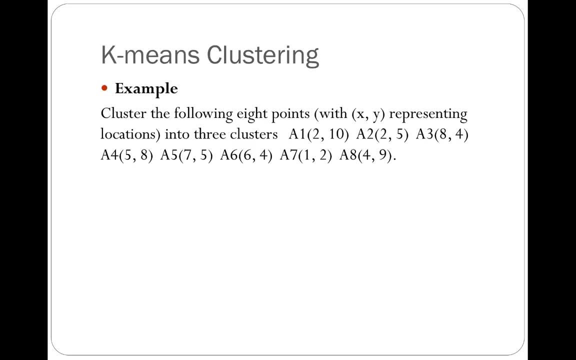 Now the question is how we define those. Sometimes we can pick three points randomly from the set of the points that we have available as the initial centers, but they don't have to be necessarily among the data points or observations that you have. In this case, I'm going to choose three points. 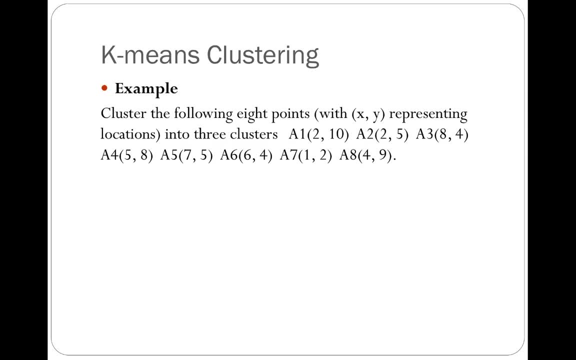 from the data set randomly as the center for each cluster. but you don't have to do that. So the center for a cluster could be totally a random number that is generated in x-y axis. But in this example suppose that we have point one, four and seven. 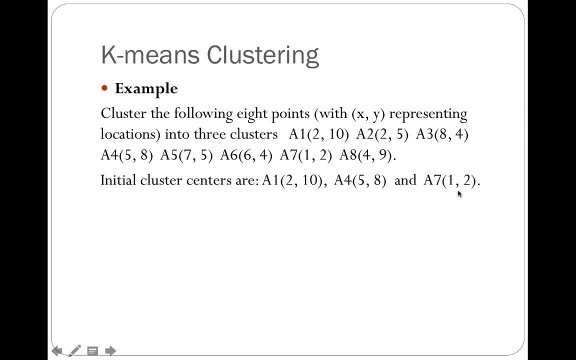 as our initial starting point. These points, as you see, are a part of the initial data set, And then we also want to use the rectilinear distances to calculate the distance between observations. Now we would like to use K-mean clustering to group these observations. 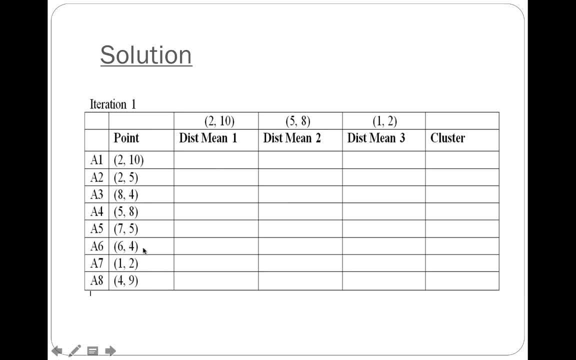 So I'm going to start by calculating the distance of all these eight points from the random initial point that I have selected as the center of each cluster. Remember, point one, point four and point seven are randomly selected to be the center of the three clusters that we have. 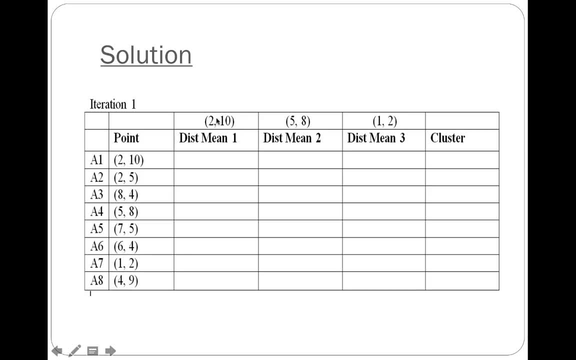 Now I have to calculate the distance of each of these points from these centers and fill out this matrix. So one important difference between K-mean clustering and hierarchical clustering is that in hierarchical clustering you had to create an eight-by-eight matrix to calculate all the paired distances. 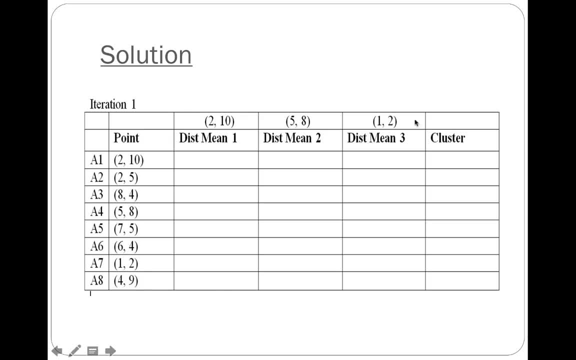 But in K-mean clustering you just calculate an eight-by-three matrix. in this case, that reduces the computational time significantly, especially when you're dealing with really big data sets. So how do I calculate the distance of two and ten from the other observation two, ten. 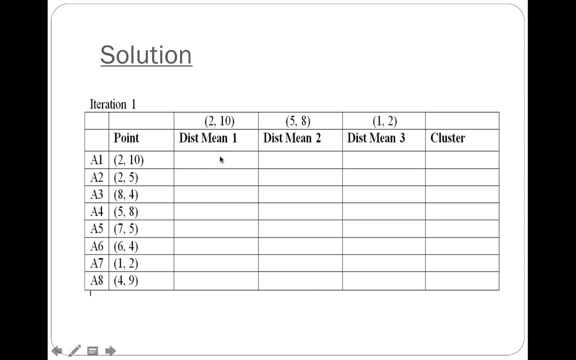 So this obviously is zero, because the distance from each point from itself is zero. But two and ten, from five and eight, simply would be the difference between the x values, which is two and five, so you have three, and the difference between y's. 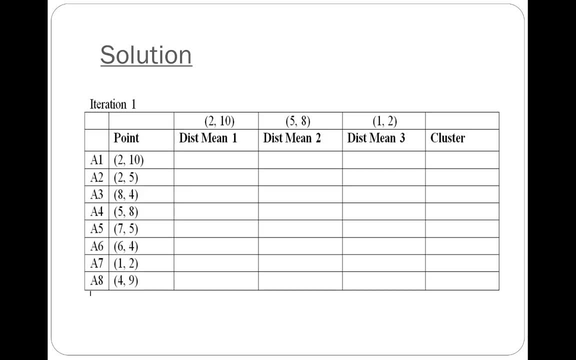 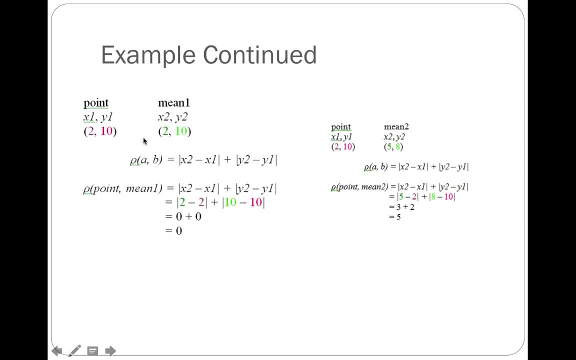 which is ten, and eight, which is two. So three plus two is equal to five. So if I want to show you more formally, as you see, the distance between two ten and two, ten is going to be two minus two. 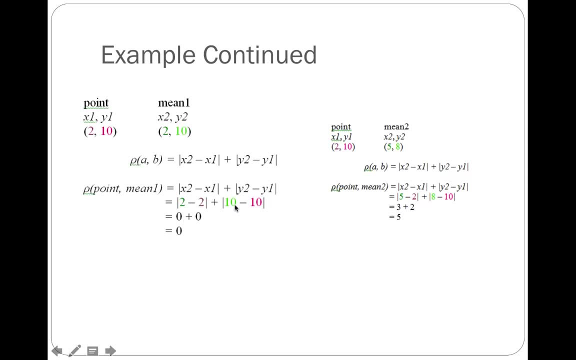 absolute value is zero, ten minus ten. y is the difference between y's and you have zero and the summation is zero. In this case, two minus five. absolute value is three. ten minus eight. absolute value is two and the total distance is five. 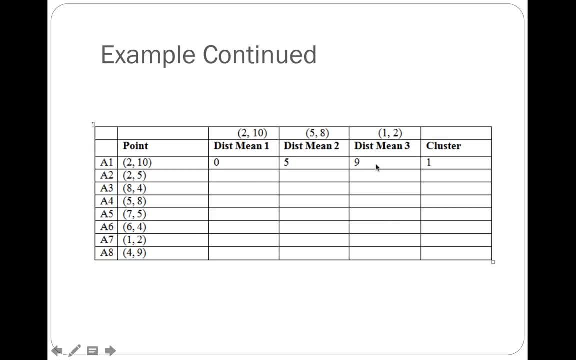 So we calculate all these distances the same way. So, for example, two, ten from one to the distance is going to be nine using the rectilinear equation. Now how can I identify the cluster for point two, ten? I have to look at all these distances. 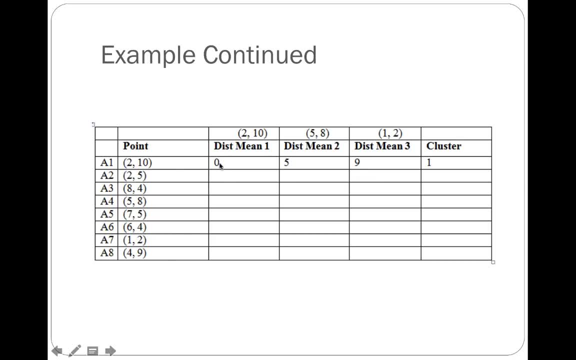 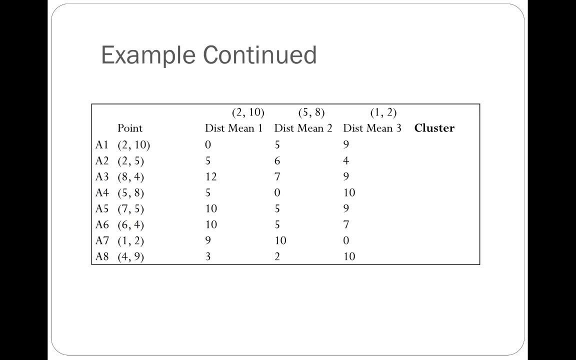 and then minimum distance would determine the cluster for this observation. So right now, the minimum distance from two ten is from cluster one, so therefore this point belongs to cluster one. Let's calculate all these distances and identify their clusters. So now, in this table, I've completed the calculation. 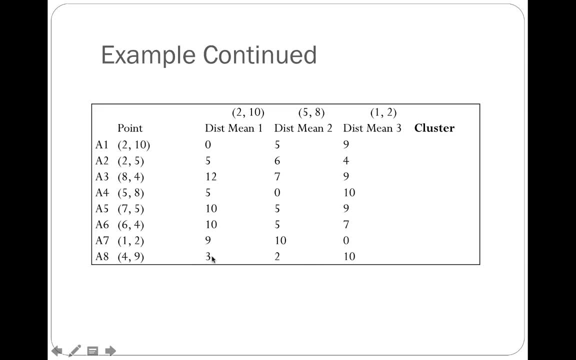 of all these distances. so any observation here, any value that you see, is the difference between the point that is given here and the center of the cluster. So now we can start allocation of all these clusters. So the closest point to two ten is two ten. 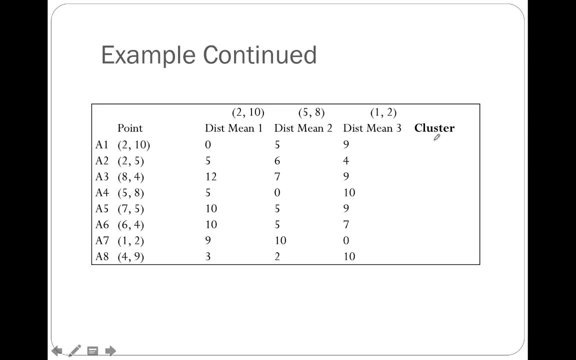 So this point belongs to cluster one. If I look at the second row, the closest distance is to cluster three. so therefore the allocation of cluster to this point would be three. So if I look at the third row, you see that the closest distance is seven. 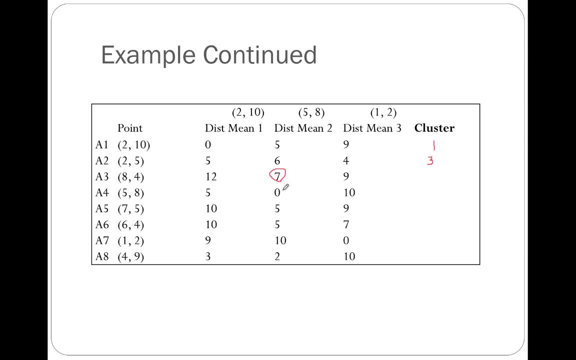 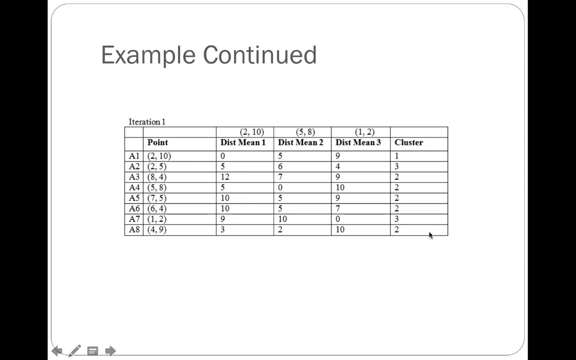 so we are allocating this observation to the second cluster. Same thing for the next row and the row after and the row after. So all these points belong to cluster two, And you can fill the rest of this table. If you do that. this is the final. 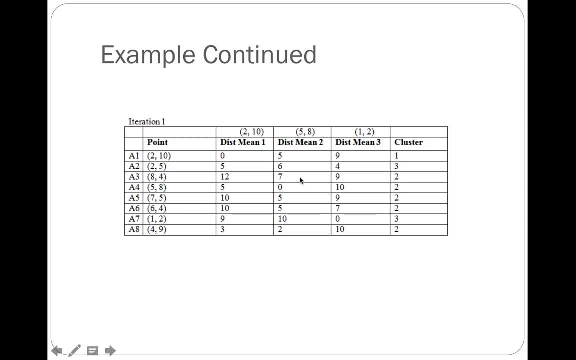 clustering allocation that you get. As you see, for example, here, the closest distance is to cluster three, so this cluster flag will be three. Now we have created the first clustering schema. It means that the first point is going to belong to cluster one. 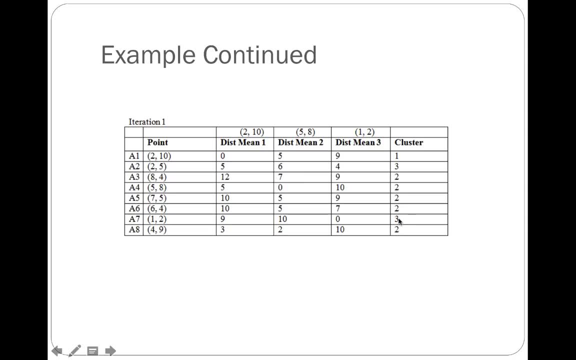 These points, plus the last observation, are cluster two, and point two and seven are cluster three. I'm going to write down the clustering schema that we have created here. Cluster one only includes two and one. Cluster two is point three, four, five, six and eight. 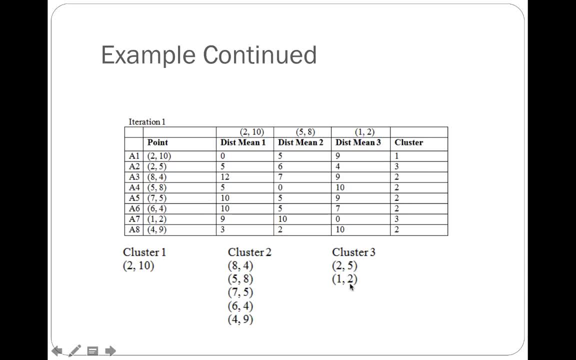 And cluster three is observation two and observation seven. Now the next step is repeating the same thing, but this time we have to update the center of these clusters. Instead of two, ten, five, eight and one, two, we're going to update the center of each cluster. 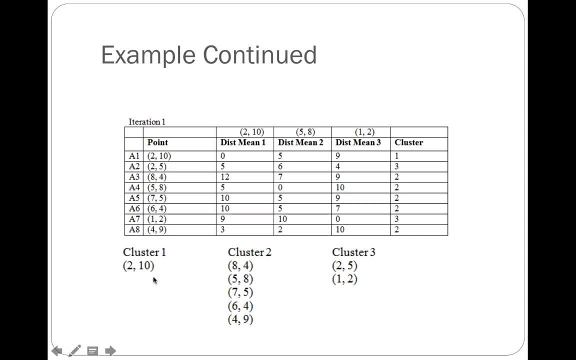 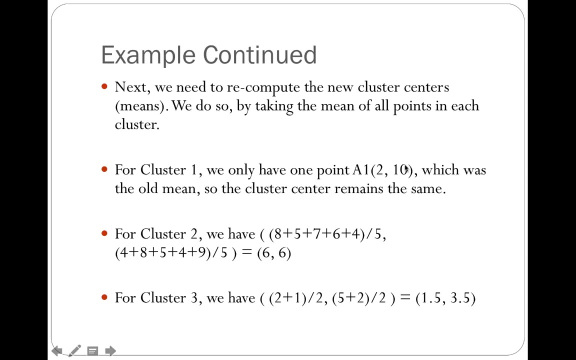 by calculating the centroids of each of these clusters. So the centroids for each cluster is simply the average of all the x's and average of all the y's. So in the next slide you see how we calculate the centroids for each cluster. Here in cluster one we only have one point. 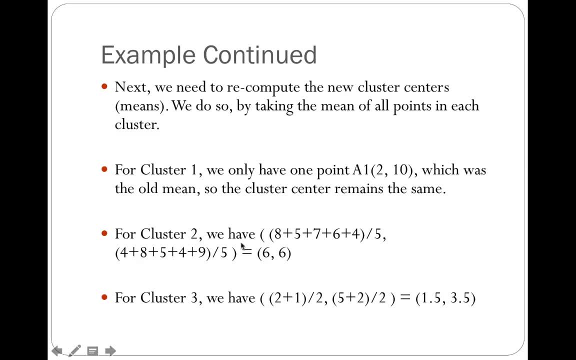 so that remains as the center of each cluster. But for cluster two we had five points. If I take the average of x's for those five points it gives me the x for the centroid, and if I take the average of y's of those points, 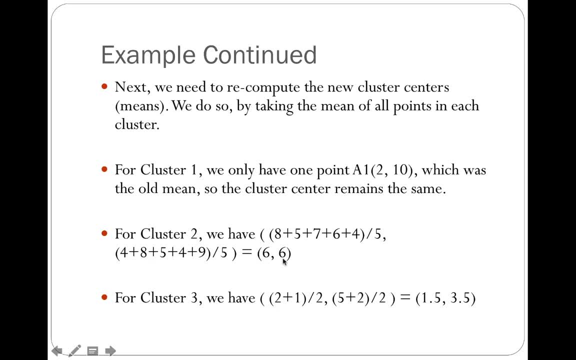 then I get the y value for the centroid. I do the same thing for cluster three. We had two observations. average of x and average of y gives me the new centroid. Now we have three new centroids: two, 10, six and six, one point five and three point five. 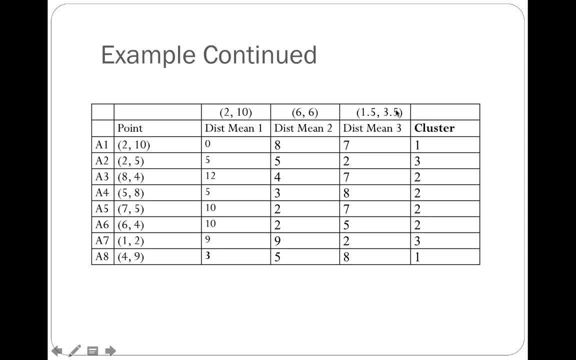 So what happens next on the top? here you see that I updated the centroids. This time the distance is going to be calculated from each observation to these updated centroids And we repeat everything exactly the same way and in the end we see which observation. 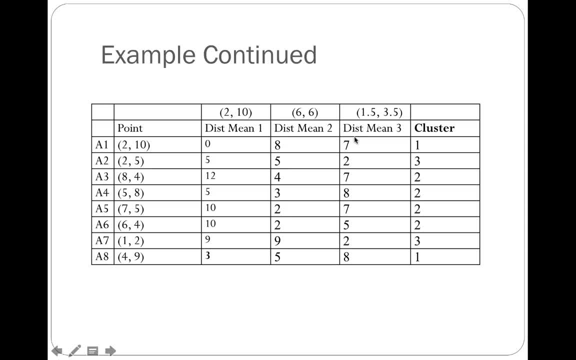 has the closest distance to each cluster and then, using that, we define the cluster in each observation. For example, first point has the closest distance to two- 10, which is the first cluster. so the cluster is going to be one. The second point, the closest distance, is to third cluster. 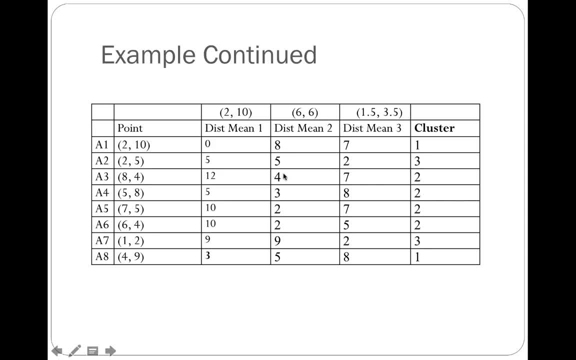 so that becomes the third cluster. This one is second, so that becomes the second cluster. second cluster, second, second, third and first cluster. So in each row you're looking at the minimum distance from the point to center of each cluster. 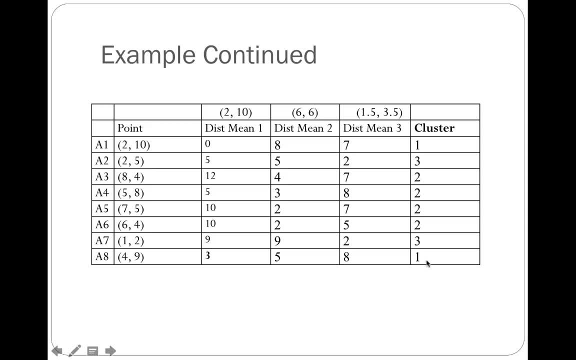 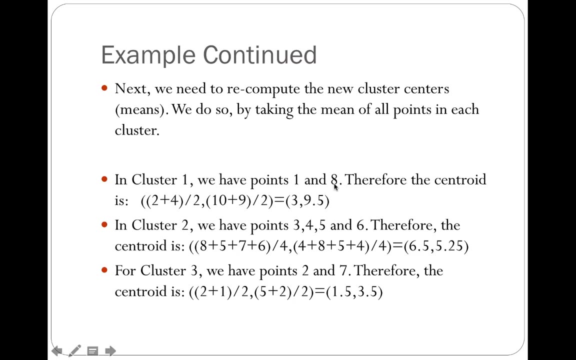 and identify the cluster allocation. Now we have to repeat the previous step one more time. We have to find out what are the points within each cluster and update the centroid for each cluster. If I do that, I see that this time point one and eight are in cluster one. 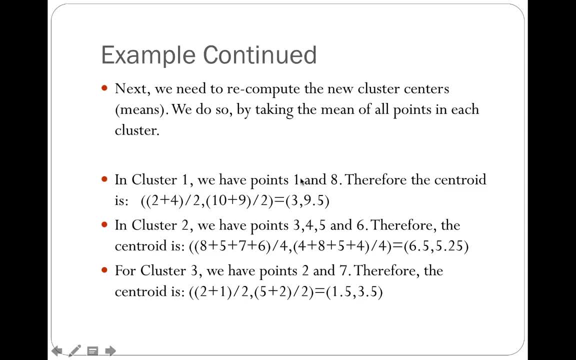 I take the average of x and y for point one and eight and this is the new centroid. Also, point three, four, five and six are in cluster two. If I take the average of x and average of y, these two becomes the centers for the new cluster two. 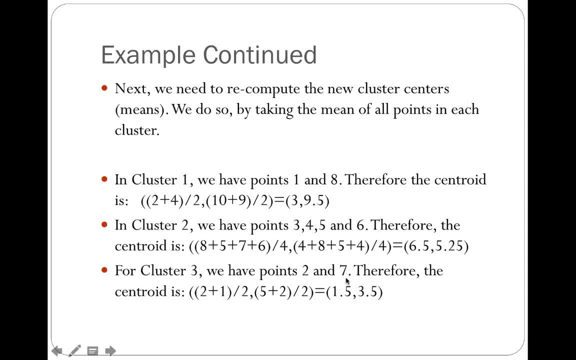 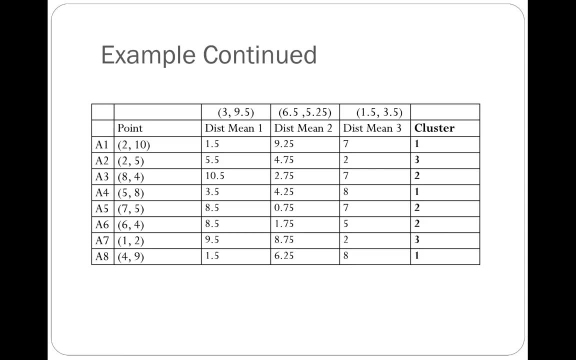 and cluster three only includes two and seven. If you update that you get 1.5, 3.5 as a center for these clusters. So we repeat this step one more time, but this time we again update the center for each cluster. 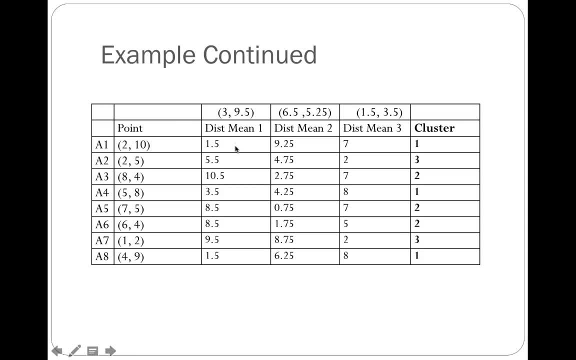 calculate the distance of each of these points from these clusters and find the minimum distance from each observation from each cluster and define the cluster schema or cluster allocation. If I this time look at the allocation of points to each cluster, I see that points one, four and eight are cluster one. 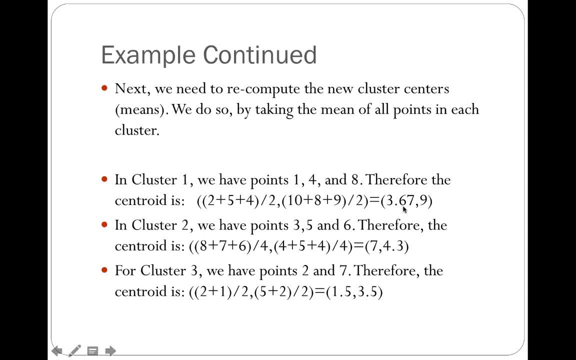 So if I update the centroid this time I get 3.67 and nine for the first cluster. For the second cluster you see three, five and six belonging to cluster two. If I update the center for the cluster by calculating the average of x and y, 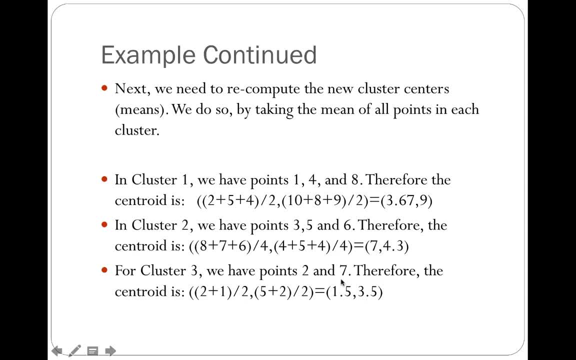 you get seven and 4.3, and point two and seven belong to cluster three. So if I calculate the average of x and y within each group, this is the new centroid that you get. Now I have to repeat that I update the centers, update all the distances. 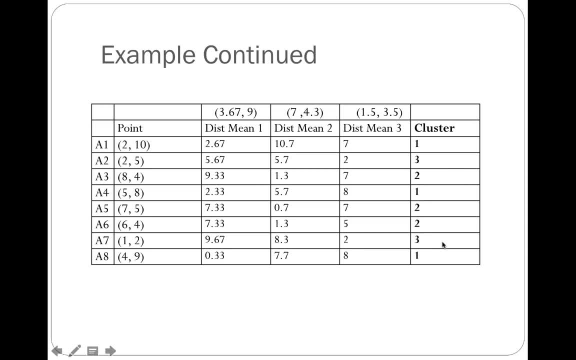 and update the cluster allocation. So if I do that, I see that I exactly get the same allocation that I got last time. It means that point one, four, eight are in cluster one, point two and seven are in cluster three and the rest of the points are in cluster two. 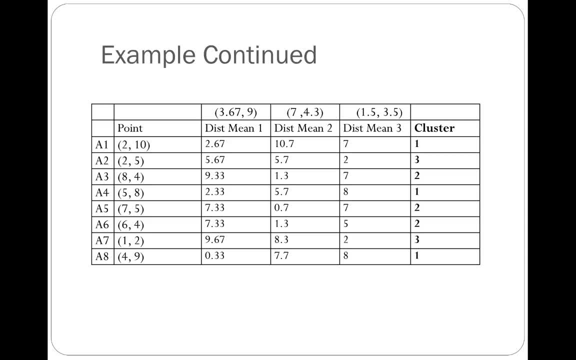 This is exactly what we got two slides earlier when we had different set of centroid. So this is a sign that we have to stop the k-min clustering and report this as a final result or as the final cluster allocation. The k-min clustering ends when your clustering method. 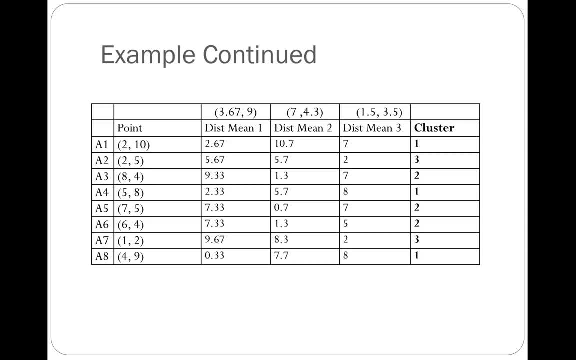 from one step or one iteration to the next one does not change. So right now you're in the final allocation. It means that point one, four and eight are in cluster one. two and seven are in cluster three and the rest of the points are in cluster two. 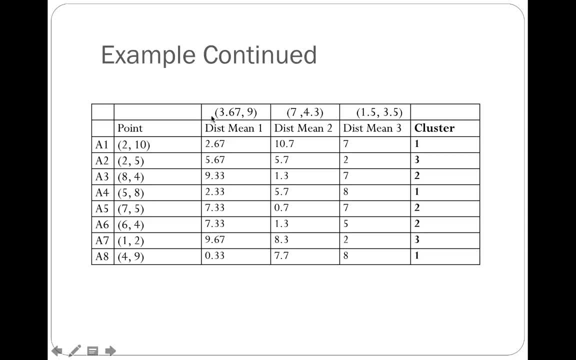 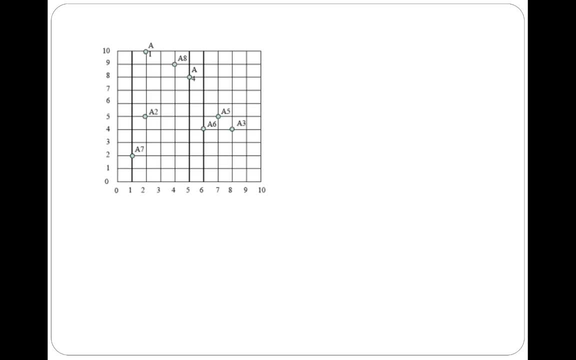 The centroids for these clusters are given on the top. This is an image that kind of shows what just happened throughout the k-min clustering with a visual graph. These are the eight points that we got. These are the points that we had at the beginning. 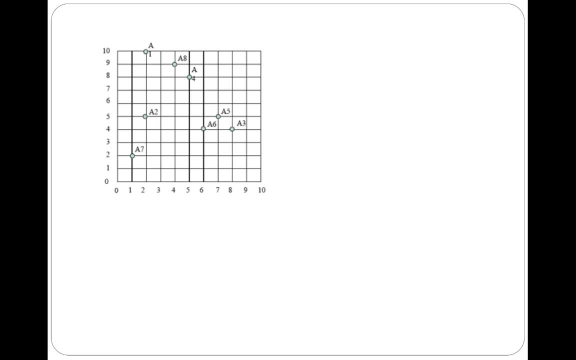 Now what I did. I started putting three points of these observations as the center of my three clusters. I picked A1, A4, and A7. Then what I started doing is started allocating clusters. find out what are the closest ones to each observation. 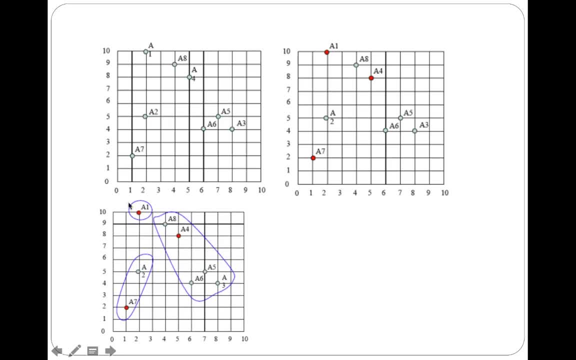 or each centroid in this case. So, if I do that, this was the first iteration that we ran. A1 was cluster one, A2 and A7 were cluster three And the rest of the points were cluster two. Now, then, after that, when we updated the centroid, 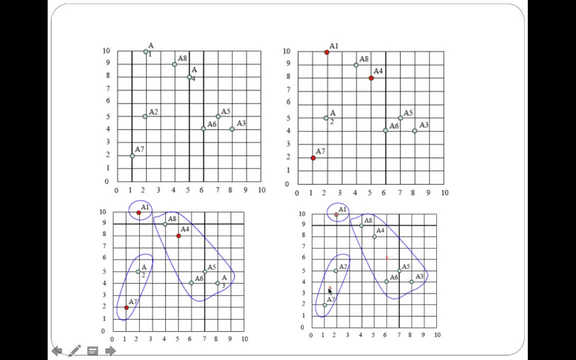 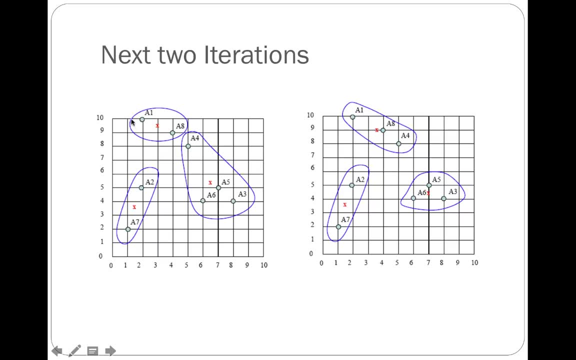 these points that are shown by red are the new centroids. So we have to repeat the allocation schema And after we did that, you see the next two iterations, A1 and A8, fall into the first cluster, Two and seven into the third. 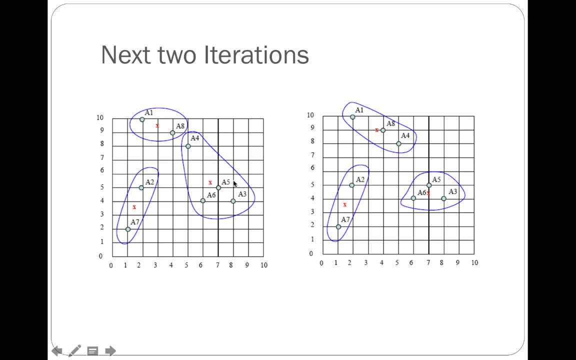 And the rest into cluster number two. When you repeat the process of finding the centroids and allocating points to the clusters, you got to the final iteration, which was here, And after that, when you repeat it, your clustering schema didn't change. 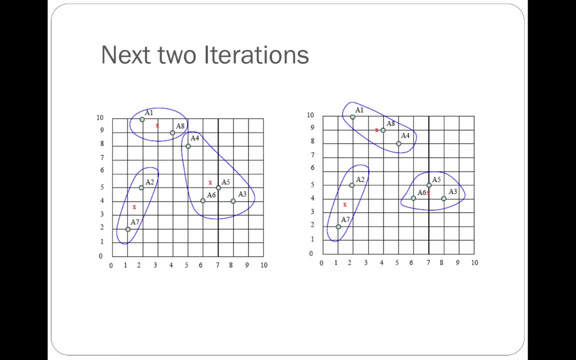 That means that you're in the final clustering stage and your clusters are formed. Now you can report your final clustering schema, which is: one, eight and four in cluster one, Two, seven, cluster three, Five, six and three in cluster. 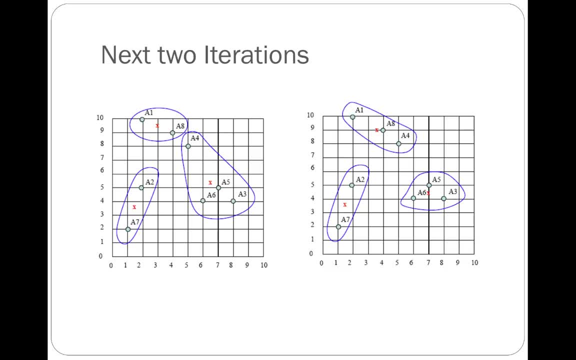 Two. With that, our lesson in clustering using K-mean method has concluded. Please refer to your Blackboard for your assignments. Thank you. 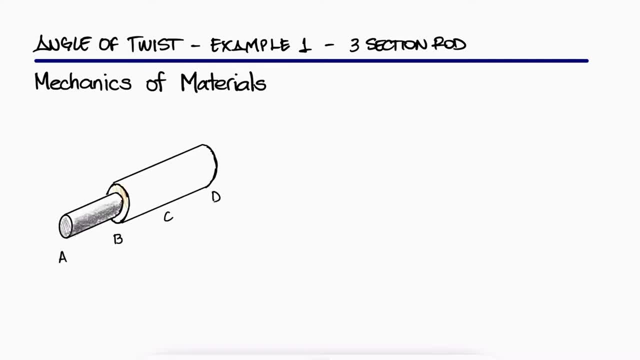 The aluminum rod AB is bonded to the brass rod BD. Knowing that portion CD of the brass rod is hollow and has an inner diameter of 40 millimeters, what is the angle of twist at A? This is the first example for the angle of twist and statically indeterminate problems. 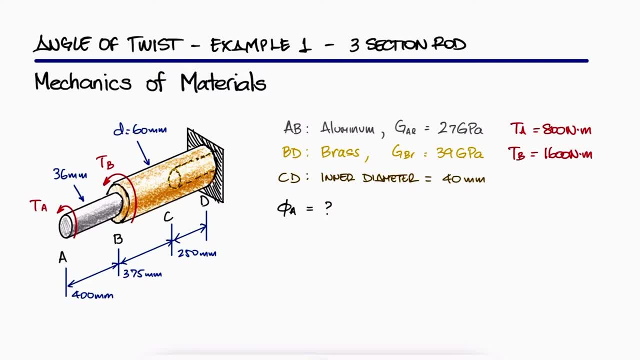 main video. The link to that video and other examples are in the description below. We can find the angle of twist at A. if we find the angle of twist of A with respect to D, which is the wall, This is the same as the angle of twist of A with respect to. 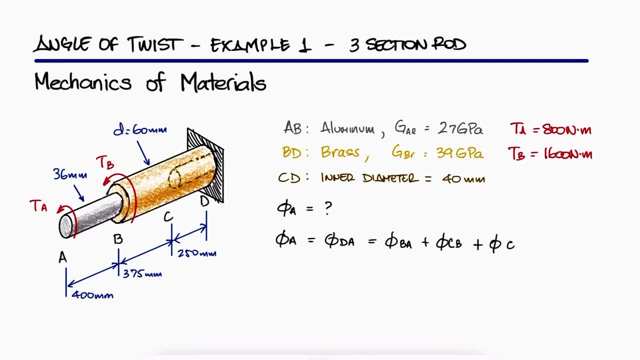 B plus B with respect to C plus C with respect to D. For each section of the rod we need to find the torque, the length, the polar, second moment of area and use the shear modulus information. The lengths are given and we know the shear modulus between A and B for 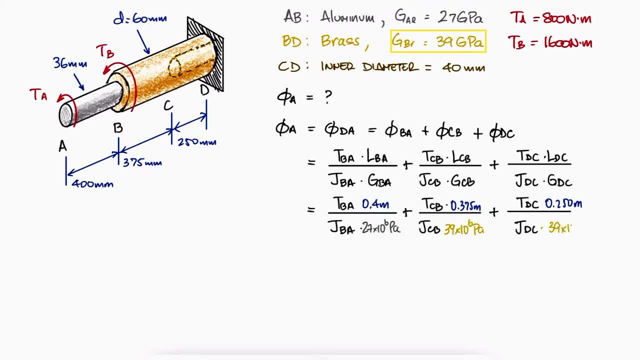 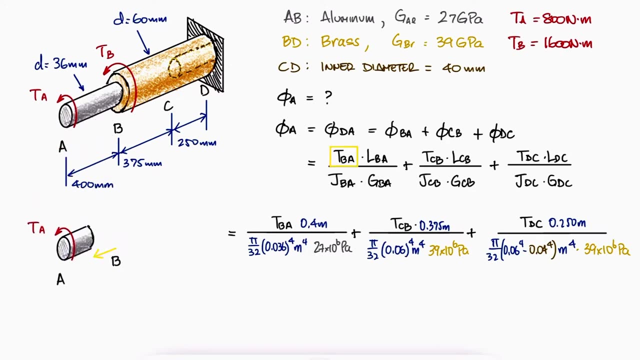 the steel and between BC and CD for the brass. The polar second moment of area can be calculated for that of a steel rod. If we have to calculate the torque of A, we need to say that the torque of A is the signal of the normal structure of the solid cylinder for A, B and BC and that of a hollow cylinder. 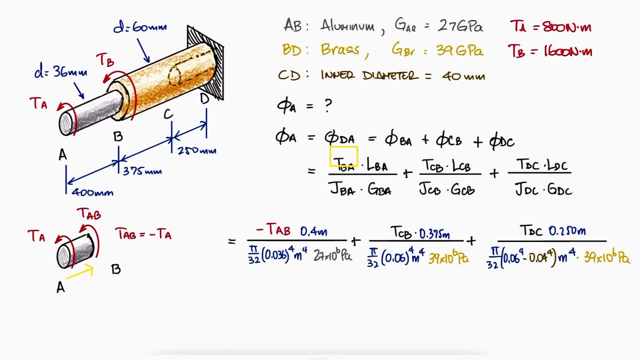 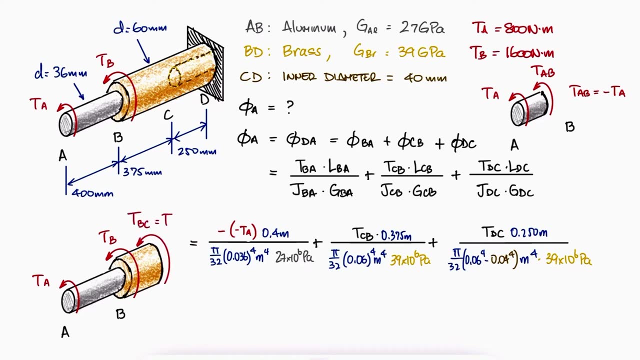 for section CD, The internal torque TBA from B to A will be the same as the negative of TAB from A to B, which means that the internal torque in the first term is just TA. The internal torques from C to B and from D to C will be the same, since there are no